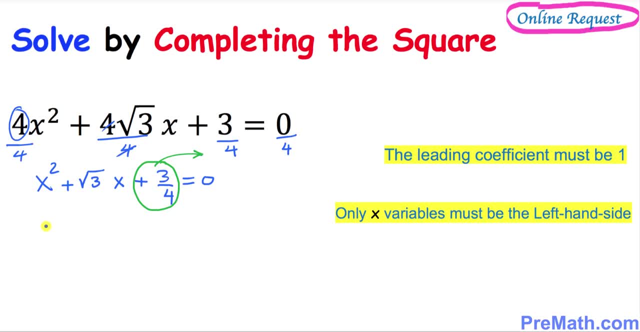 right hand side. So what we're gonna get is we have simply x square plus square root of 3 times x, and when you move this positive 3 over 4 on the other side becomes negative 3 over 4.. Now the next step is I want you to just 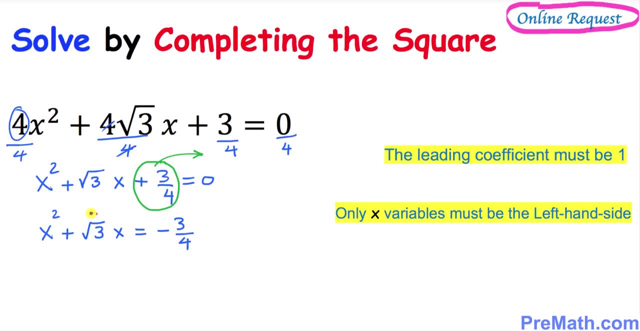 focus on this part. the coefficient of x. Don't worry about this sign, only this thing. I want you to write it down Over here: square root of 3, and the next step is: I want you to divide this one by 2.. Always divided by 2, and then the next. 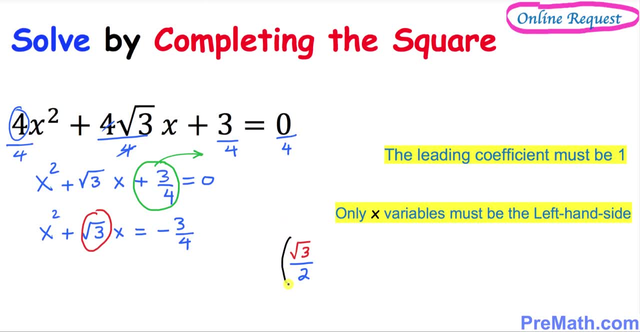 step is: I want you to take the square of this one, All right. So that means whatever we got this thing over here, we're gonna add this quantity on both sides, So 1 over 4 plus 2 would be x squared over 4.. So this means we separately. 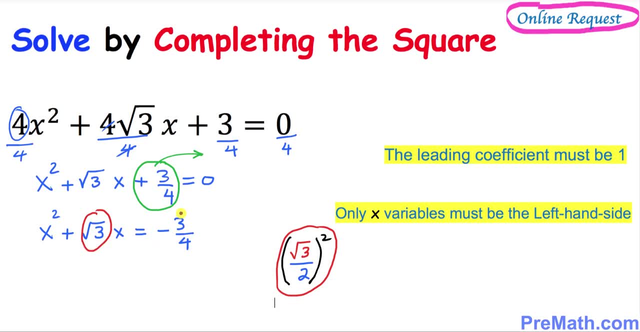 both sides of this equation. so let's put down like: x square plus, square root of 3 x plus, equal to negative 3 over 4 plus, and now we are going to add this quantity on both side, which is square root of 3 divided by 2 square, and on this side, 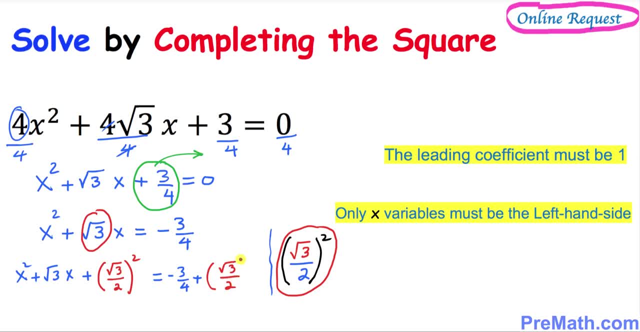 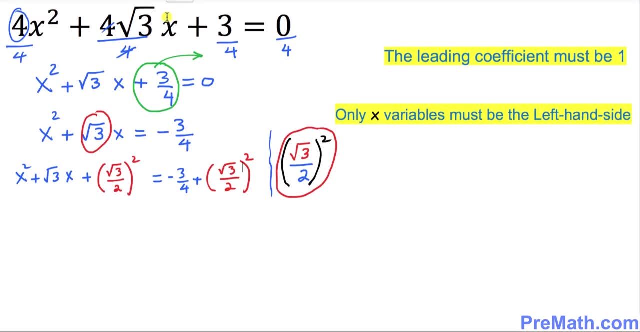 square root of 3, divided by 2 square on both sides. so far, so good. now i want you to look at this side, this part over here. on the left hand side. this represents a complete square of x plus 3, square root of 3 over 2. 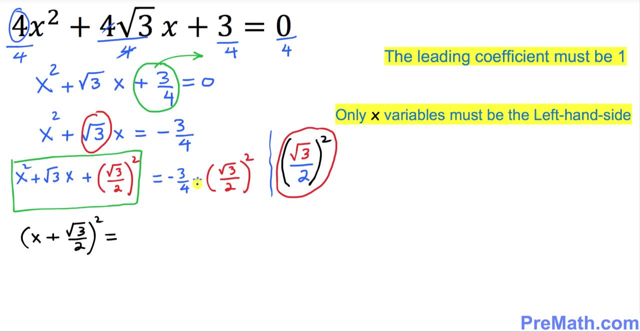 square equals to this on the right hand side is negative: 3 over 4 plus. and when you take this square, you see this, this one over here. square and square root- they undo each other. we got 3 over 2. square is going to be 4. that means what we got is x plus. 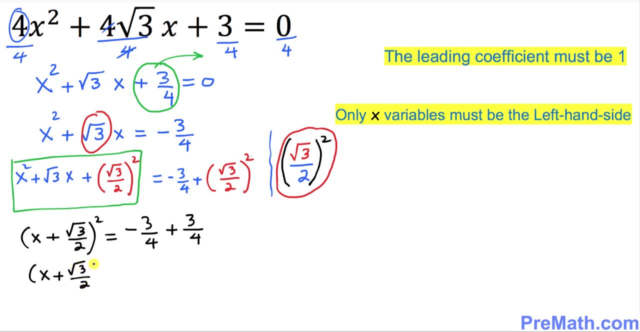 square root of 3 divided by 2 turns out to be equal to 0. and if you are wondering, how did we get from this point to this one, over here we use this fact. over here you remember, always remember, a square plus 2 times a, b plus b, squared always equal to a complete square of. 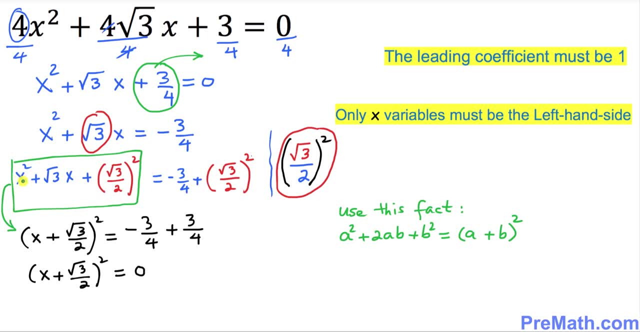 a plus b, power 2.. so over here, this is what we got. x turns out to be over here, showed up right here. whatever in this parentheses, it showed up right up here. and whatever this sign over here, this comes over here, all right, so we are pretty sure that we're able to compute this. 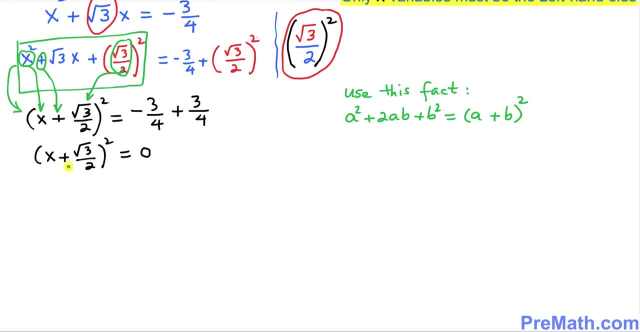 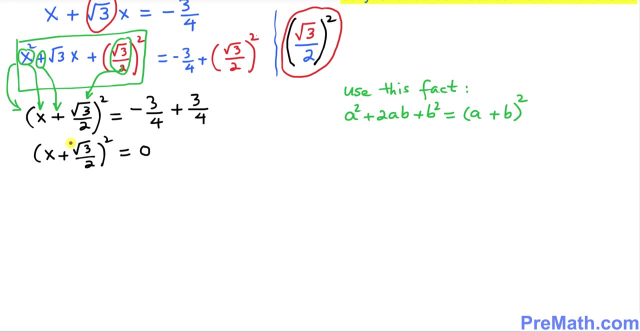 much done over here. we wanna isolate X. as you see, we must get rid of this square, so we're gonna take care of, we take, take the square root on both sides. so this square and square root, they undo each other. we got X plus square root of. 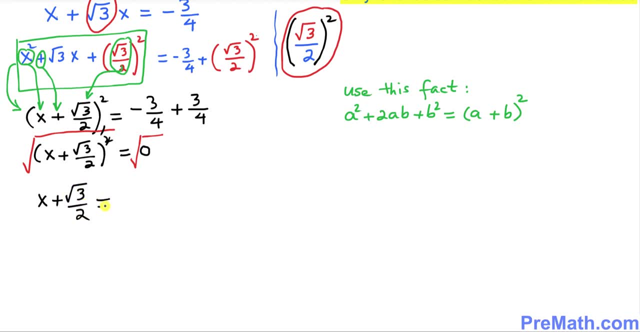 3 divided by 2, equal to square root of 0, is always 0, but make sure you put down positive or negative 0. now, since we want to isolate X, we must move this one, this quantity, on the other side. so we simply got X equal to negative square root of. 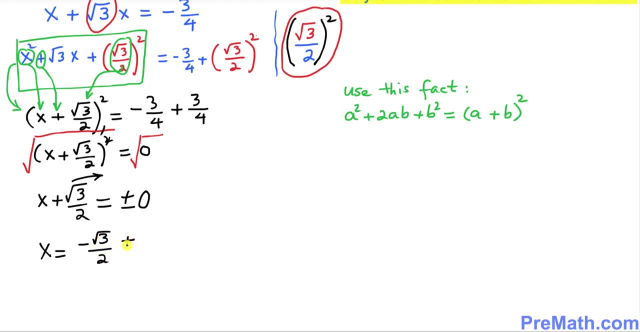 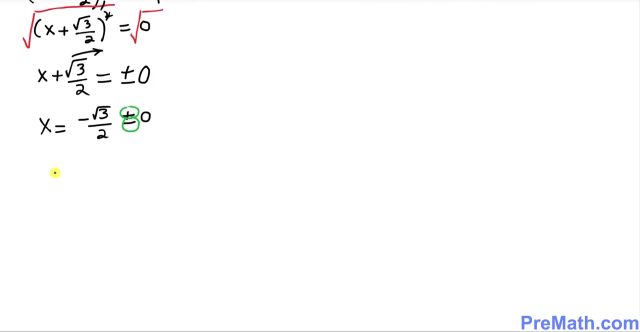 3 divided by 2 plus or minus 0. so we are going to split these signs up positive and negative. so let's go ahead and take care of that thing and we will be pretty much done so. first I'm gonna put down negative square root of 3 divided by 2.